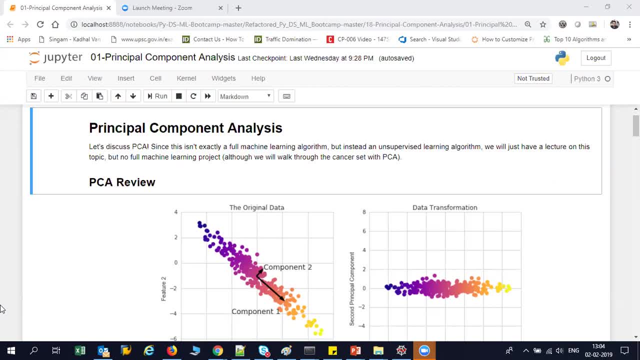 dimensions and then you can apply your machine learning algorithm. Always remember that. it is always said in machine learning that as the number of dimension increases, so there is always a curse. So as the number of- sorry, as the number of dimension increases, as the number of dimension increases, then it is. 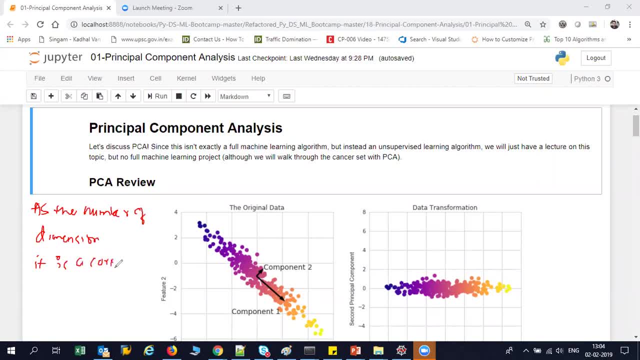 actually it is a curse. Reason why we call this is that always your accuracy gets impacted with the number of dimensions. If our dimension increases, your accuracy gets impacted. If this dimension increases, your accuracy will become less. Now let us just understand a small intuition behind how this principal component analysis. 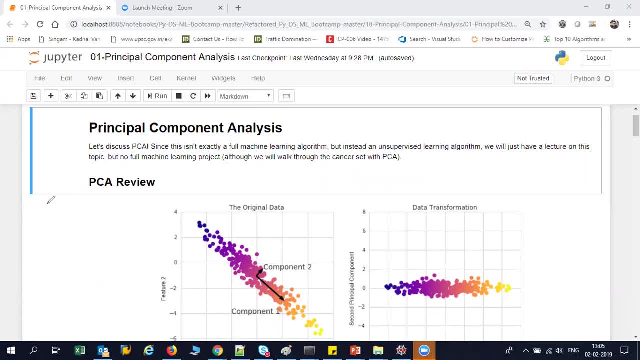 works. So, first of all, let us consider that I'm going to show you a two dimension feature and I'll try to convert it into one dimension. So we'll try to understand what are the will be used in order to convert a two dimension into one dimension. so let us just continue. let's 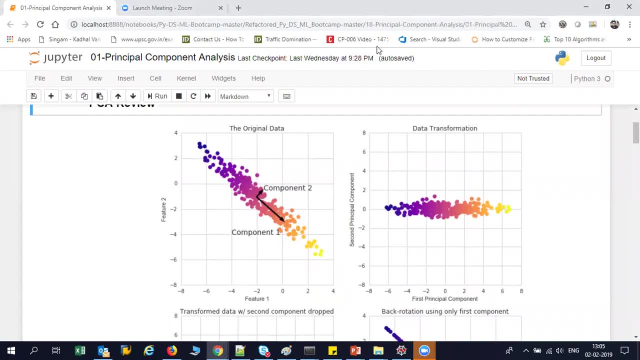 let us just understand the first first part, that is, the intuition part. so to begin with, suppose i consider that i have a two dimension. two dimension that is basically two features, that is, this is feature f1 and f2, and some of the points are populated somewhere like this: 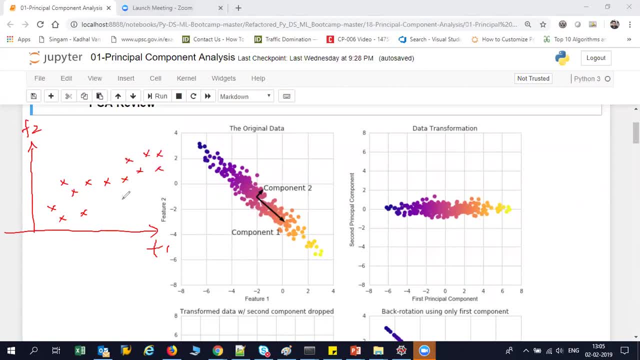 right now, when i see this kind of features, right, i want to convert this into one dimension. when i say that i need to convert this to this two dimension feature into one dimension, that basically means that i need just a single line, because this is basically my one dimension. 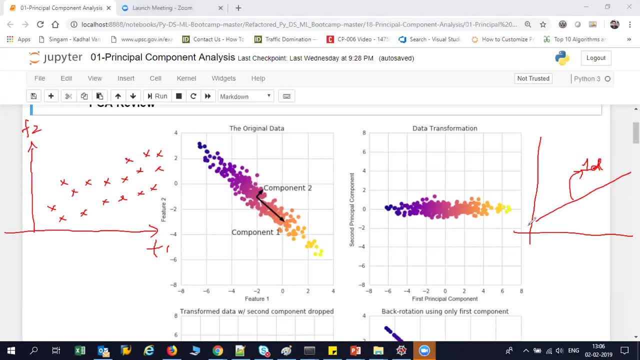 link right. it is just like a one dimension. now in i have to project all this point in this particular single line. so how do i do it? so the first step is that we actually try to calculate the best vector space which can represent as the best fit line. 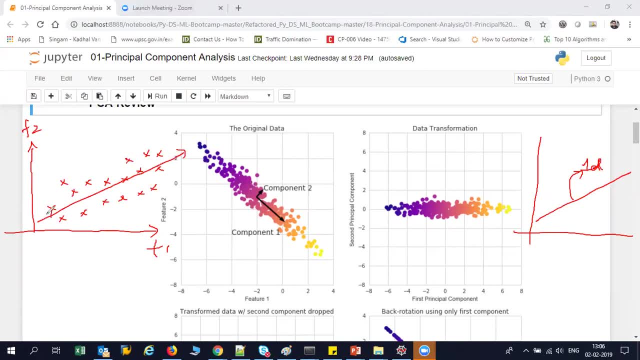 for all these points. the next step, basically, that we do is that we try to project this point. we try to project this point, not going much into the mathematical equation, but this will definitely help you out how this particular line is actually created, which line we should actually consider as a one dimension line. now, when we project this line right, you can see that. 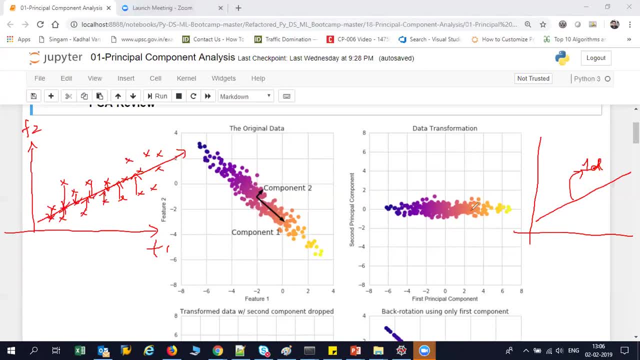 my new features will be this point, and this, in turn, is actually forming us, this particular line. now you may also have a scenario. you may be asking, krish, why, why can't we just consider other lines too from this? why can't we just consider the other best fit line? so usually what happens is that, first of all, when i create this, 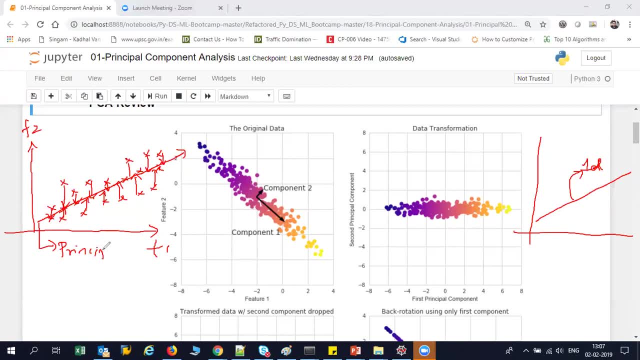 line. this line is basically called as principal component one, and you can create any number of components. but one thing that you have to make sure is that suppose the next component that will be created, it will be created perpendicular to the first line. so perpendicular basically means it will be on 90 degree or it will be orthogonal to the first line. now when i say orthogonal, what? 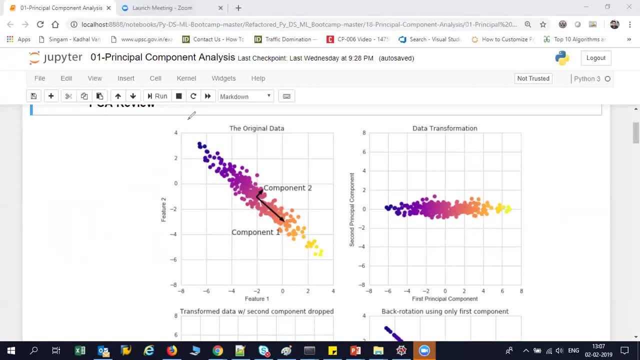 will happen, is there? so let me just draw the diagram. uh, very nicely again. suppose this is my sorry for the diagram, okay, so suppose this is my x and y feature. suppose these are my points and i i showed you that i'm i'm creating my first principal component line, something like this: 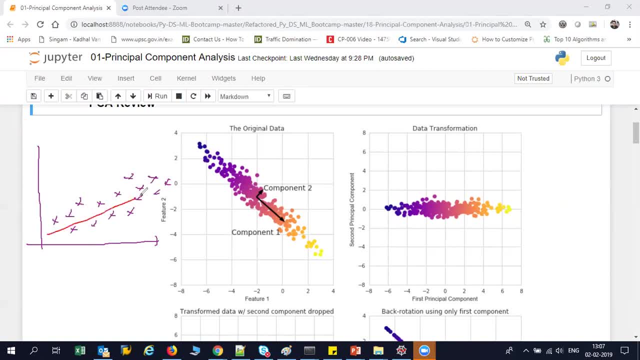 and i- i showed you that i'm i'm creating my first principal component line, something like this: this is my first principal component line and i try to project all this point at this particular location, right on this particular line, projected all this point in this particular line when i 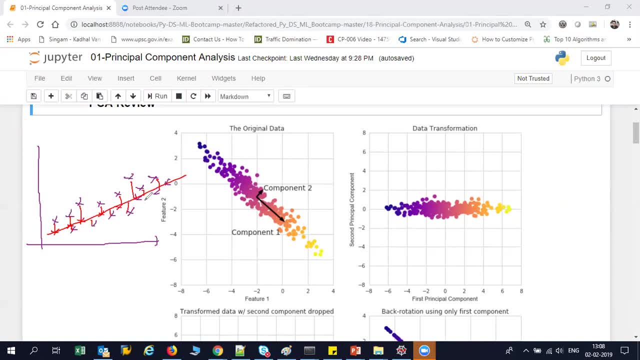 projected it. this is my new points that has got created right now. after this, what i do is that i'll create my another principal component, so this is basically called as principal component one. i'll create the another principal component, and the best technique to create is basically: i have 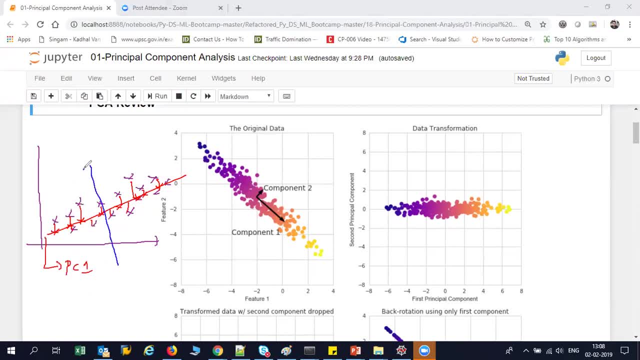 to create a diagonal, i have to get the orthogonal line. so this orthogonal line is my another principal component, that is pc2. i'll tell you why i'm creating it. okay, so there may be a question like: why should we just select this particular line instead of the other lines? so now, when i 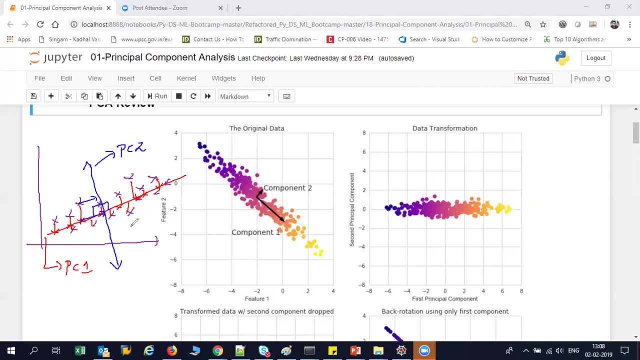 just try to plot or project this particular point over here. okay, i'm projecting all these points here, all these points here right now. when i try to project all these lines, you should always remember that there is a lot of variance that has been lost while projecting lost of variance. 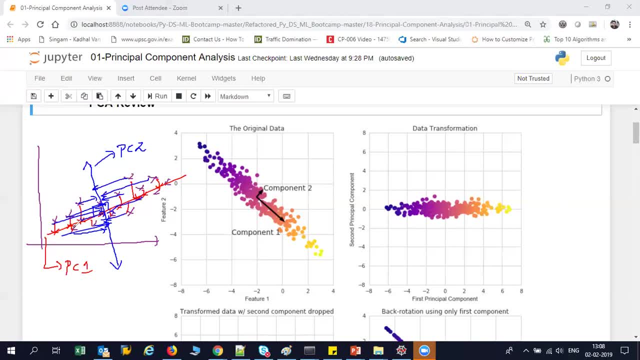 basically means a lot of information from this point. so usually, whichever information, whichever points when i'm projecting to the vector space or this principal component, at that time you should remember that there should be less number of variants or information lost. if there is more information lost, i should never select that particular now in this particular space, when i'm 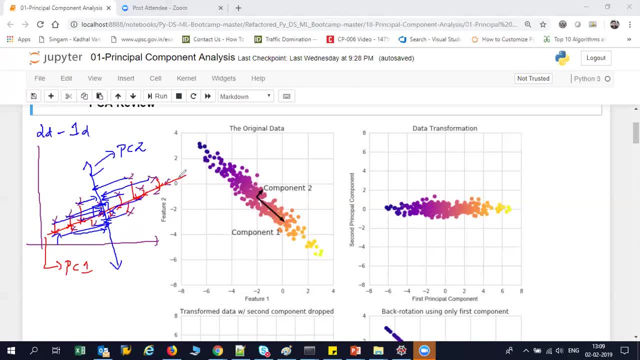 projecting all this information to one dimension to one dimension. i'm considering this line. the reason i'm considering this line? because when i project all this point right is less in number of information. now let me just consider the right example over here. suppose i create my, i create my. 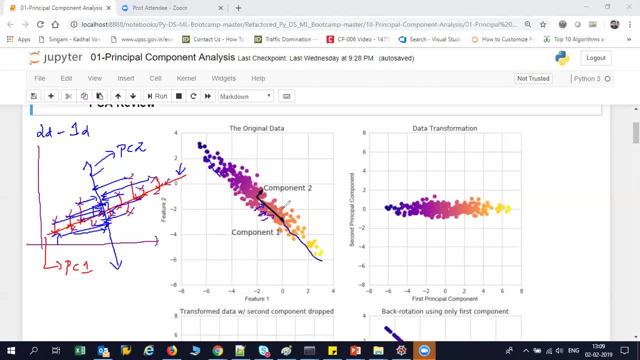 vector space like this. i extend this okay, and i project each and every point right, so there is very less information that is getting. now. suppose if i created a orthogonal line like this and i try to project all this information at this plane, then there will be a lot of information lost. 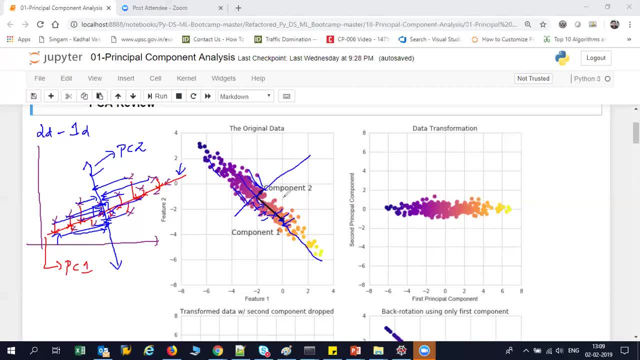 right when compared to this line. so what we do is that from this two vector space, either i can choose component one or i can choose component right now. similarly, what will happen, suppose, if you have many dimensions, like 1000 features? i'll try to create these components many times, you know. 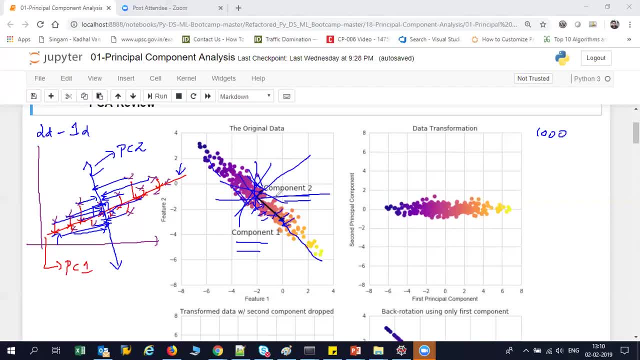 and all will be orthogonal to each other. with respect to the dimensions, and finally, i'll try to convert this into: suppose, if i'm selecting into 100 dimension this, this lines that i see over when i'm projecting, the best hundred lines will be chosen where the variance lost is very, very less. yeah, so, after i apply this particular principle component, 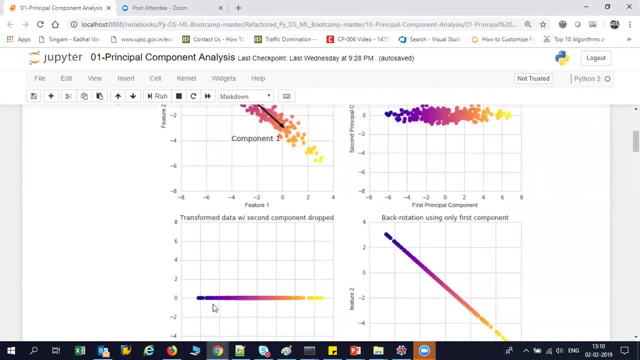 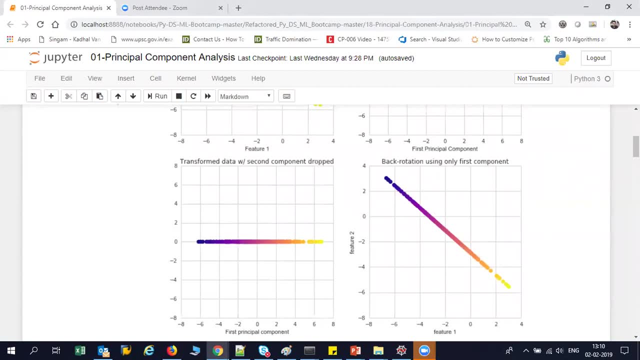 analysis and if i go and see when i see my two dimension getting converted into one dimension, it will look something like this: yeah, now let us just go and understand how we can implement by using python and skillen. so first of all, i'm importing some libraries like matplotlib, pandas, 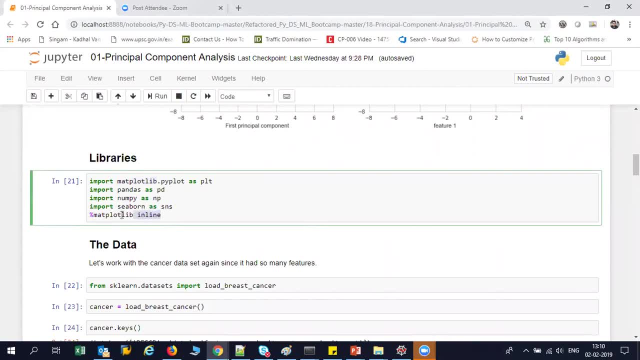 sorry, numpy, seaborn and matplotlib inline so that i can display my plot curve class within this particular jupyter node. so here, pandas is basically used for reading the data set. numpy is for creating multi-dimensional array. seaborn is used for also doing some visualization stuffs, considering statistics in mind. so i'm going to use an inbuilt. 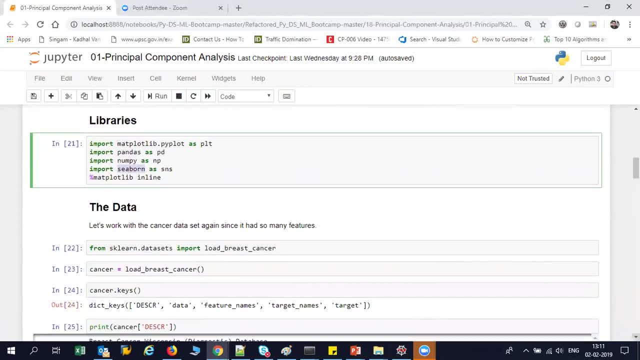 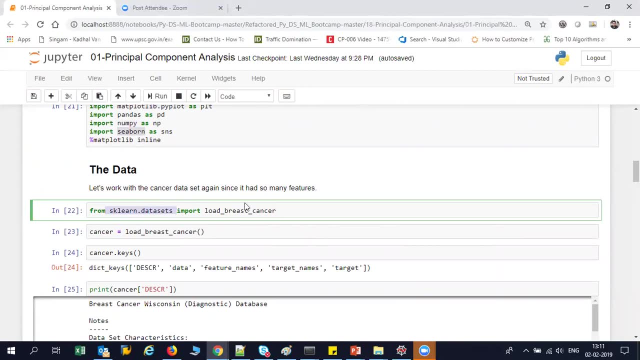 data set which is called as breast cancer data set, this breast cancer data set and that is already present inside sklearndatasets, so it is available in the sklearn itself. so i'm importing this particular load underscore- breast underscore, cancer- and i am uploading- i'm uploading the particular data set in my variable that is cancer. now, when i see cancer, this cancer will be a. 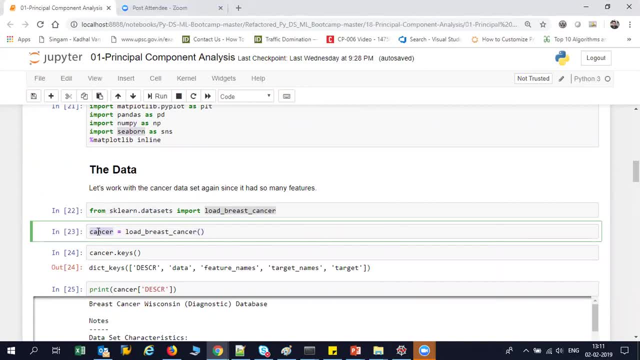 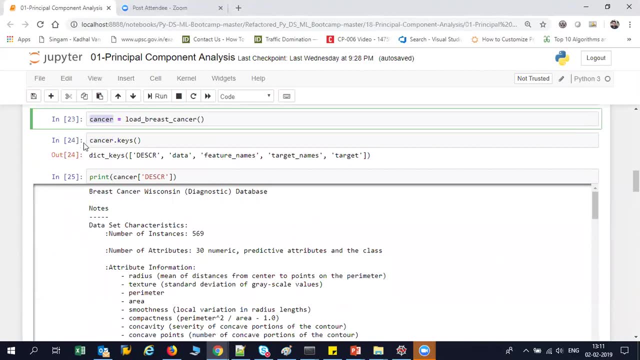 dictionary key pair. i mean it will be a dictionary values which will be having key value pairs. first of all, i'll go and see the keys. so keys over here are basically, if you just write cancer dot keys then it'll you'll be having information like description, data, feature name, target names and. 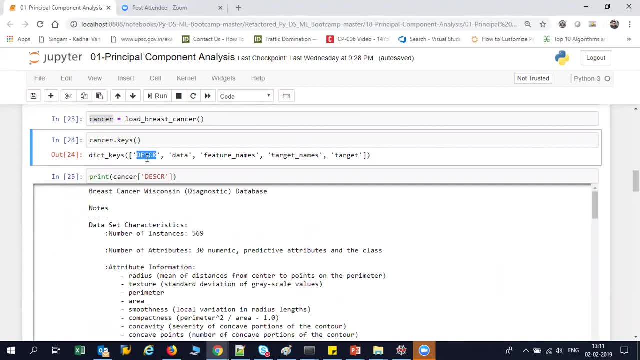 target right now: this description. if i go and try to understand this description, you will see that all the information about this data set is given over here. see this: i'm writing print cancer of description as my key now. if you go and see the information about this data set, all the 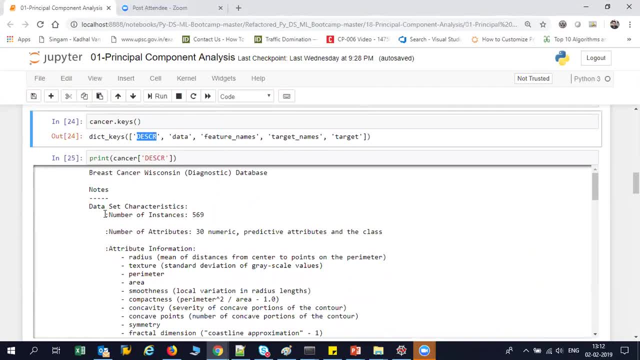 information will be present inside this dictionary. now over here you can see that some of the information is number of instances. this is basically the number of records. so the total number of records that i'll be having is basically 569. the total number of attributes is basically. 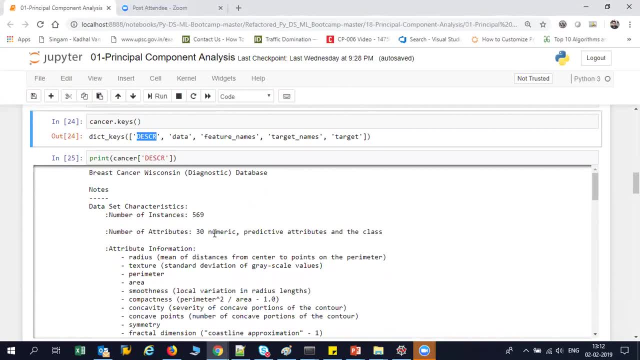 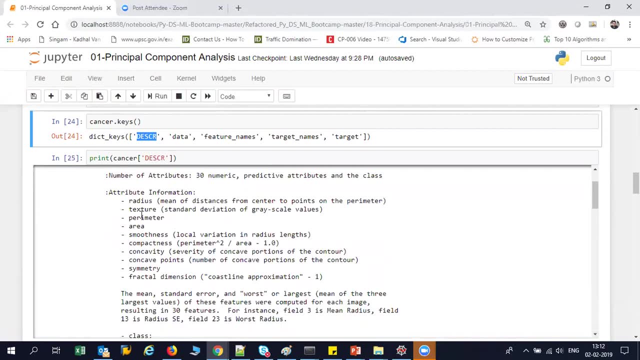 30 attributes, or this. attributes basically means the number of features. now, what are the feature of this data set? so this is the information that we have. let's go and see. so we have something like a radius, texture, perimeter area, smoothness, compactness, connectivity, contact point, symmetry. 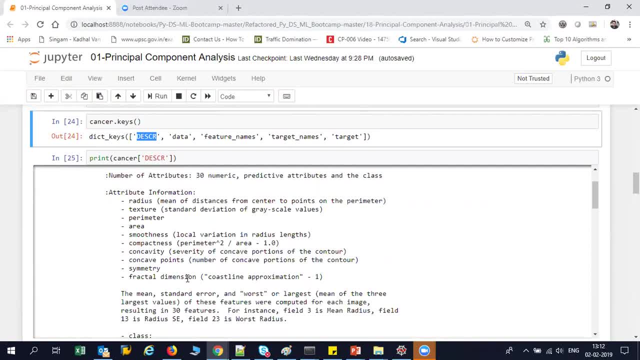 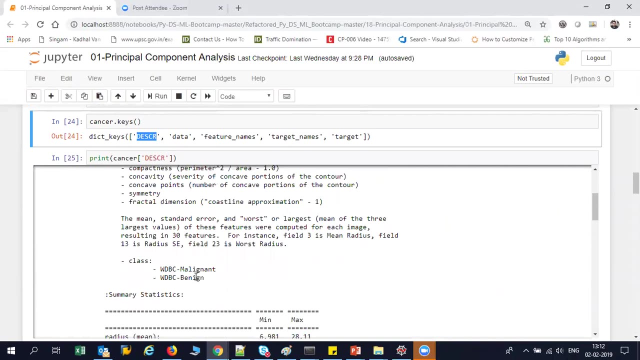 factor dimension. again, guys, this information is all about the size of the tumor. okay, various sizes of the tumor that is actually responsible for causing the cancer, cancer disease. and if i go and see my target types, how many different types of target i have. so i have two classes. one is 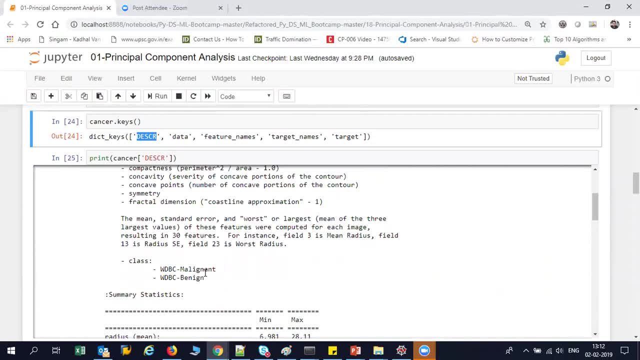 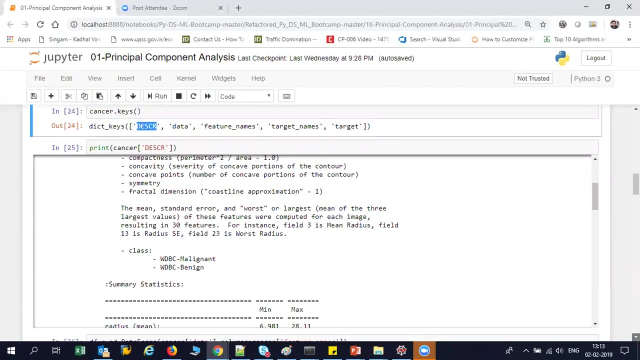 malignant and one is benign. so i have two outputs, or two outputs with respect to the data set. with respect to all these features, i may either have malignant or benign cancer. okay now, if i go down. okay, so only two types of cancer may occur from this particular data set. okay, now, if i go, and what i'm going to do is that, first of 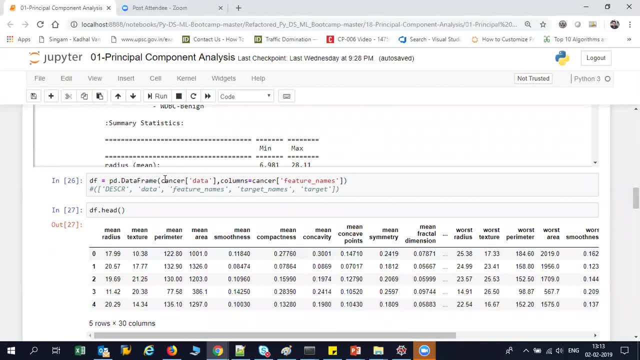 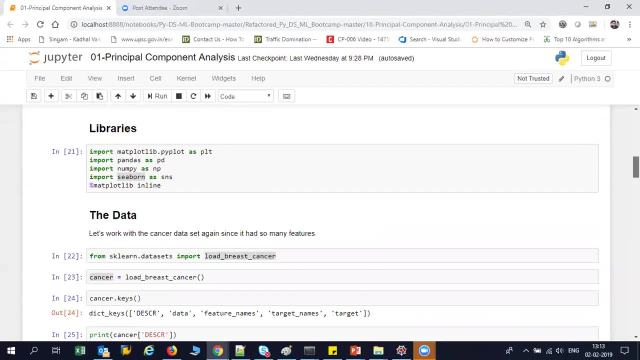 all. i'm going to create a data frame where all my data i'm taking as all my data, my column name should be the column of features name. now you can see that on the top i have a feature names, which is called as. this feature name will basically be the name of all my columns that is used within this. 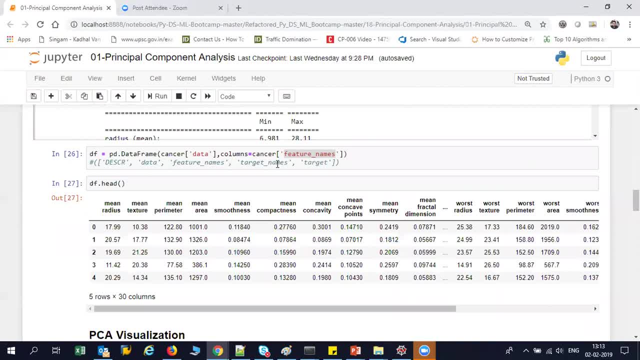 the attributes. okay, so that i'm going to take it over here and you can see that i've formed a data frame by using pddata as soon as i see the data framehead. this is how my data set looks like. i have various features and total number of features are around 30.. i've already told you, and it is. 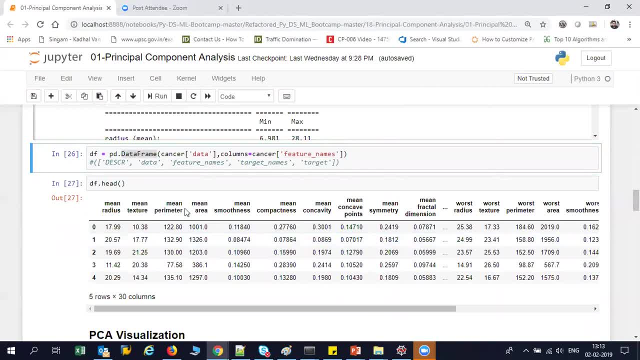 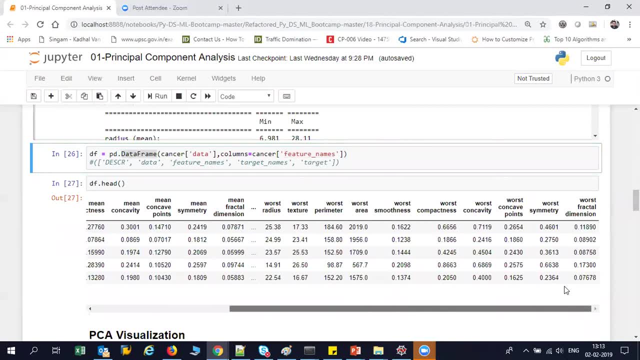 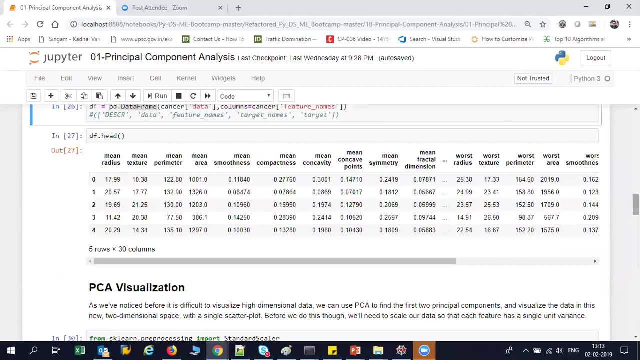 they are like mean radius, mean texture, mean parameter, mean area, mean smoothness, mean compactness. and this is the area where i have all my data points. all these information are present. so here is all the information. now the next thing is that i will try to do some visualization, but always. 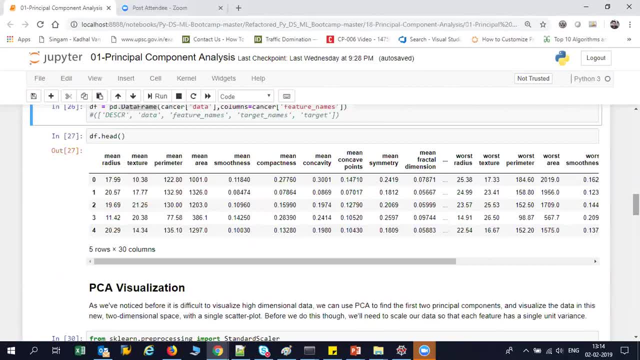 remember before i do, before i apply the principal component, analysis, to reduce the dimension over here, the total number of dimensions are 30.. from this total number of dimensions, from 30, i'm going to convert into two dimensions and then i'm going to plot that particular graph and see whether 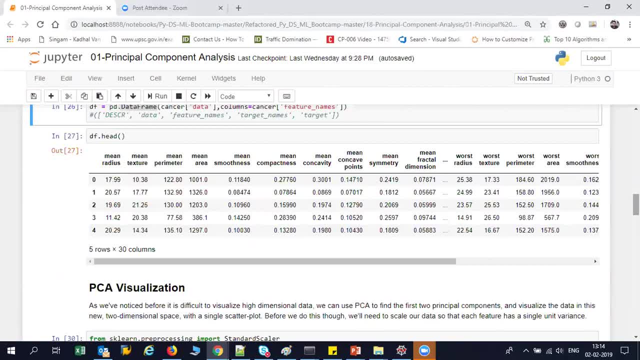 my output can be easily categorized. First of all, always remember the first step in demonstrated reduction is basically to do standard, standard normalization. Standard normalization basically means that suppose I consider all this, all these features, as my random variable. Okay, So I'll consider all this. 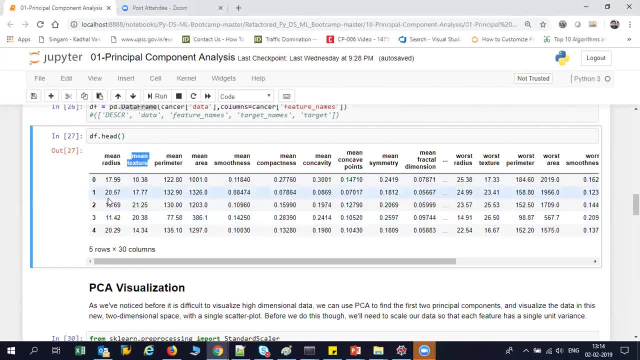 This is my separate random variable. This is my separate random variable, And if it is following a distribution which is called as Gaussian or normal distribution. because if you don't know about Gaussian and normal distribution, uh, I've already created a videos on making you understand the statistics concept and see it from a playlist or I'll. 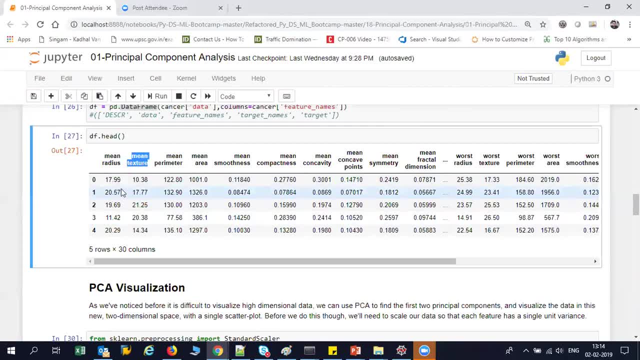 also provide a description. I'll also provide the URL in the description. with respect to this particular uh information, we'll try to convert into another distribution. wherein, wherein, suppose, if I consider mean mean radius, I'll convert this into another distribution, D dash, such that you know this. 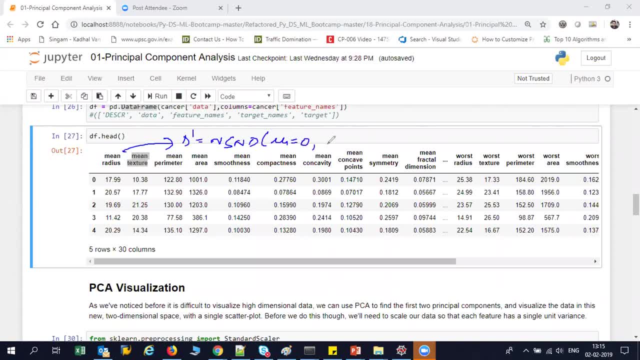 will belong to a standard, normal distribution where your mean will be zero and standard deviation. So this, all parameters, this, when, when I consider this particular feature right, This has to go through one equation which is like X of I minus mean of mean of this. 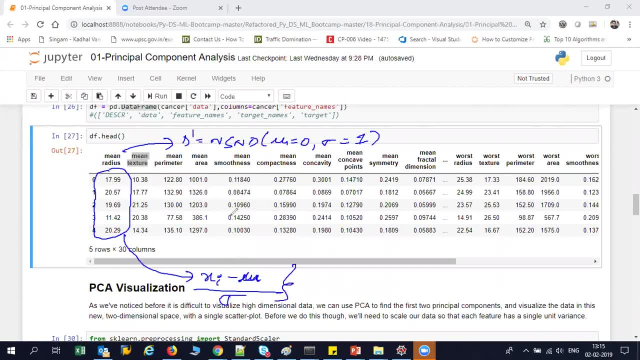 particular column divided by standard deviation. If I apply this formula, it will get converted into standard normal distribution, where my mean will be zero and standard division will be one. So I have to pass all these things and that is basically in in a scale and it is called: 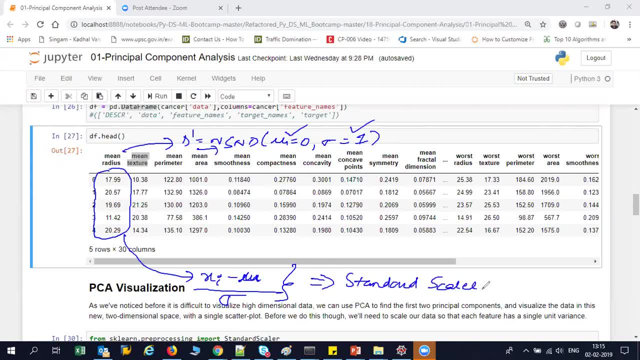 a standard scale, a standard scale. So the main purpose, The main purpose why we are doing, is because this value may be in different, different units and we need to rescale all these values in the same unit. We need to rescale the value, rescale- very important term- rescale all this value in. 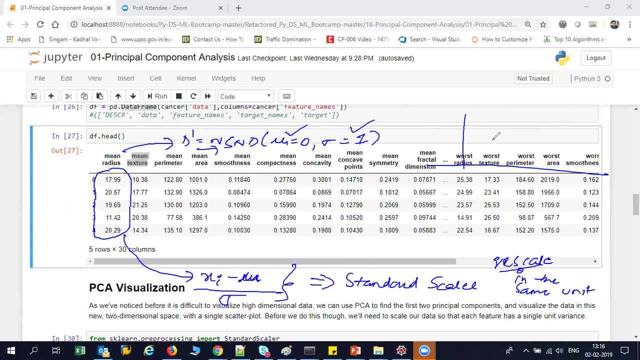 the same unit. Once we rescale, then my distribution, when I see over here it will be- everything will be very, very nearer and compact to each other. Okay, There will be no much distance, and and I, I too, don't know where this all made- 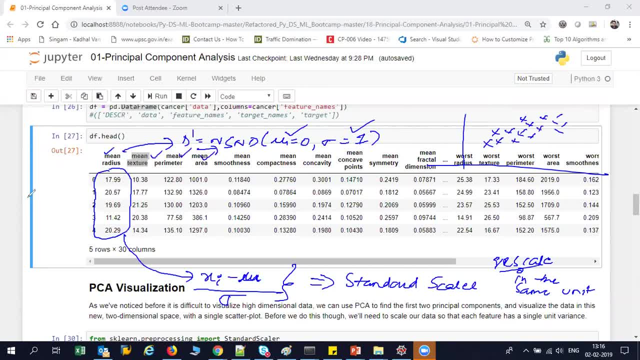 Again you say: just because the aim is to get over here misunderstood me at all And it was only right officially. but if you are in a very separate unit, like all of their fields, like your table, but no compare, you get your data from your table, you get the. 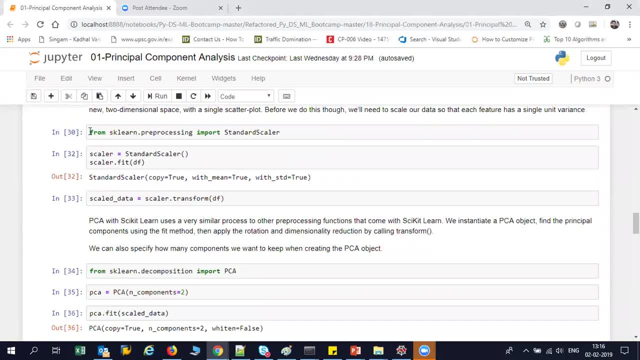 data from your table. As you can see here. see all of your data is getting separated. neighbors, you get information in this table, So we need to. how we are making this table all right, So we will go and actually make it into a all of the fields that we are using to make. 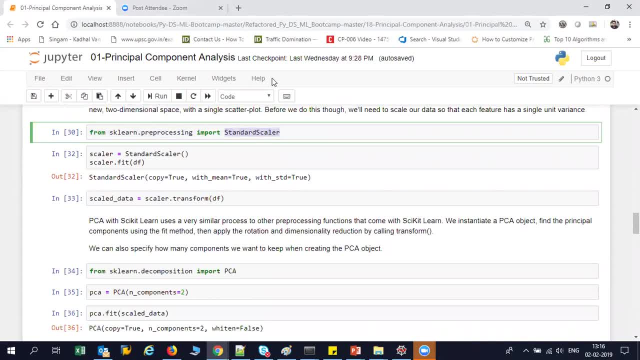 design variables: Okay, and standard deviation equal to 1. the formula that is basically applied is basically like this: X of I minus mu, divided by standard deviation. this mu is nothing but mean. this is nothing but standard deviation. but we have libraries, so we don't have to worry about it. so what? 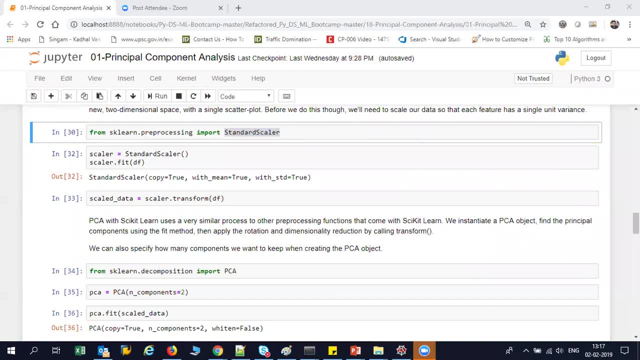 we do is that next thing that we do is that, after initializing the standard library, standard scalar, I'm going to initialize this. after importing it after good, I'm going to initialize it and then I'm going to perform fit, fit on my data frame, because all my features I want. 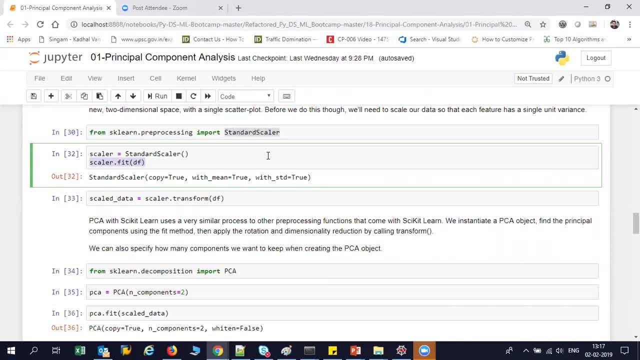 to apply and I want to convert into. sorry, I want to rescale those values into the same scale. after doing fit, I also have to apply transform, so as soon as I apply transform, all my values will get converted into the same scale. now the next thing is that: how? 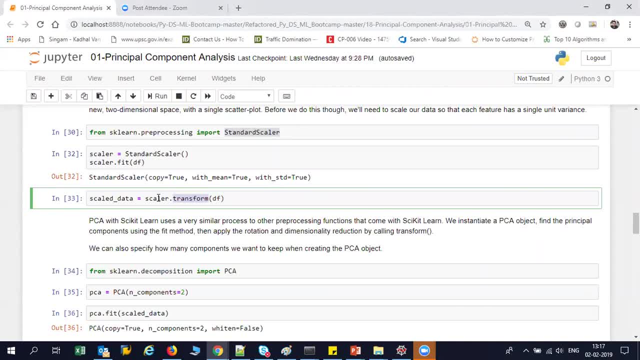 do I apply my PC algorithm again? I am telling you, it is not a machine learning technique. further PC algorithm, now PCA, will be responsible, Responsible for converting our number of dimensions, That is, 30, into two dimensions. So what I'm going to do, first of all, 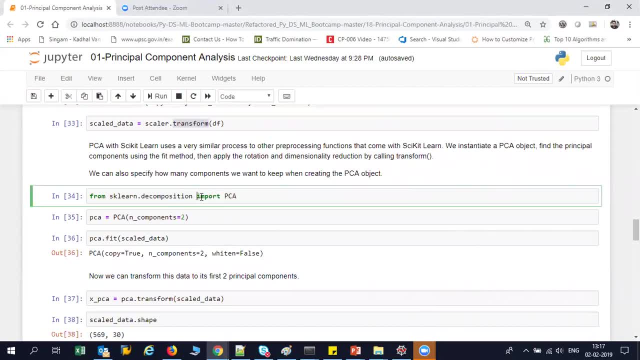 I'm going to import a scale and or decomposition. I'm going to import PC. Inside this PC, when I'm initializing it, I'll be having a feature which is called as n. underscore components is equal to 2 here. basically, I'm specifying 2 because I wanted to convert my 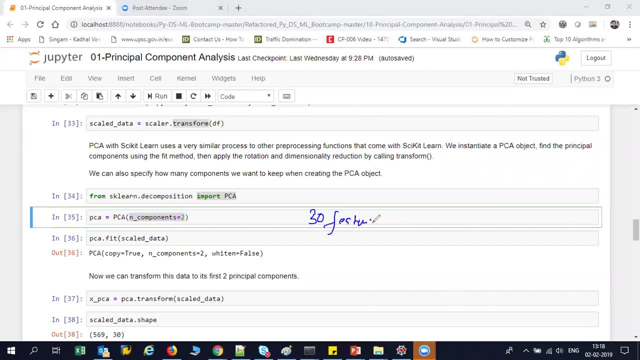 30 features, 30 features into two features and Into two features. So I'm I'm writing the same components, value as 2. Suppose, if you want to convert into three features, you can also write three. Okay, any number of features that you write, it will get converted into that number. 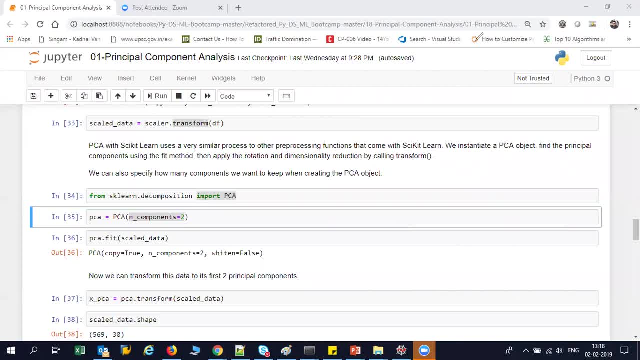 So here I'm using this and PC and then it is getting converted. then finally, I'll do fit After doing fit. okay, I'm doing fit on the scale data and you have to do on the scale data right, Which I have already scaled it down. 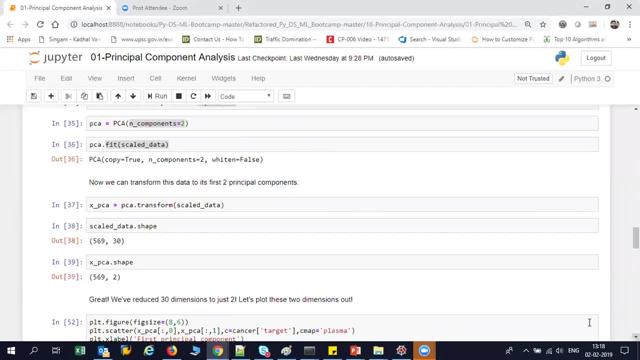 Then, after I apply fit, I'm also going to do the transformation. And as soon as I do the transformation- this is my new variable guys I'll see very important. I know my scale data, my scale data. Let's check the shape of my scale data first of all. 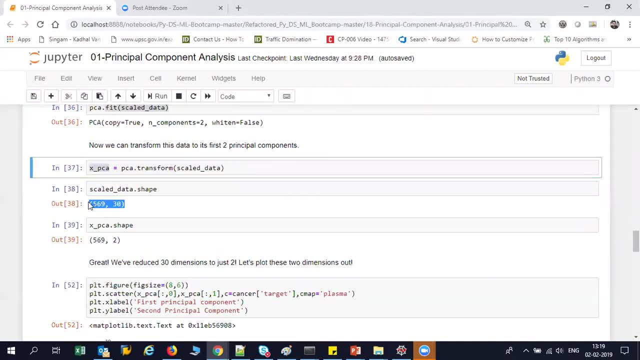 So my scale data dot shape is basically given by this particular value, by 69 comma 30, What is 569? 569 is the number of records, 30 is the number of features. now See, after I applied transform to my scale data, I got the very 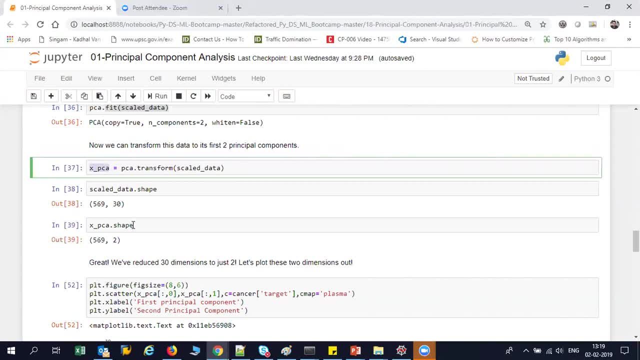 variable X underscore PCA. now this X underscore PCA dot shape, if I do, I'm having 569, comma 2, so this 30 fixed features has successfully got converted into two features. Now, still, I'm not showing you how that distribution looks like. now, if I have two features, I can actually 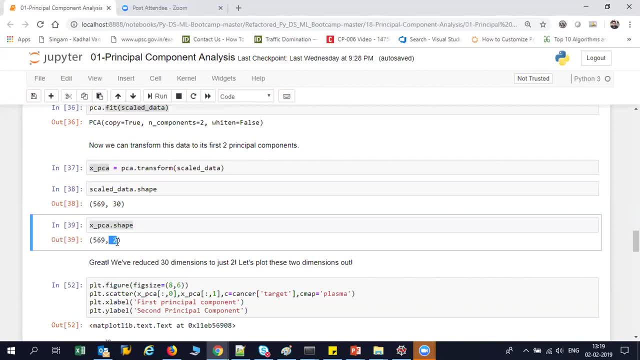 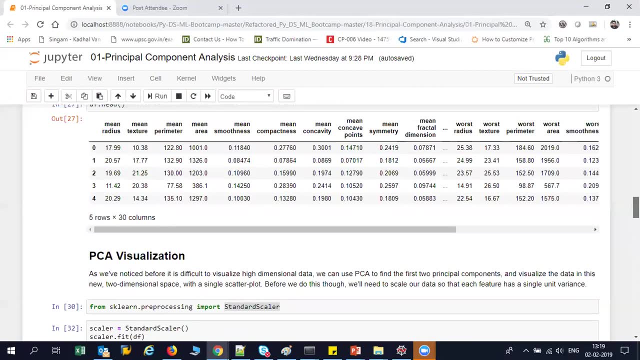 You know, create a matplotlib diagram and show to you that. how does it? how does the distribution look with respect to the output? My output is basically two features that we have Already seen in the help section. it is either malignant or benign, So let us just go and plot this particular thing. 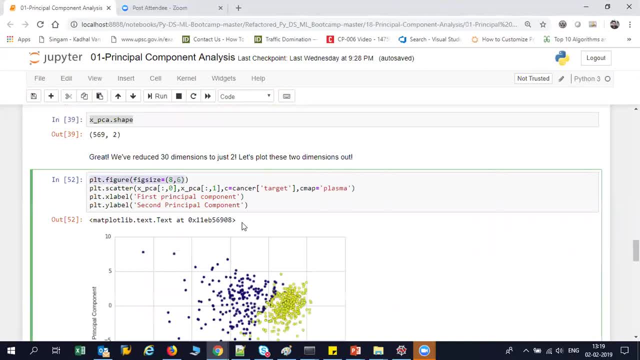 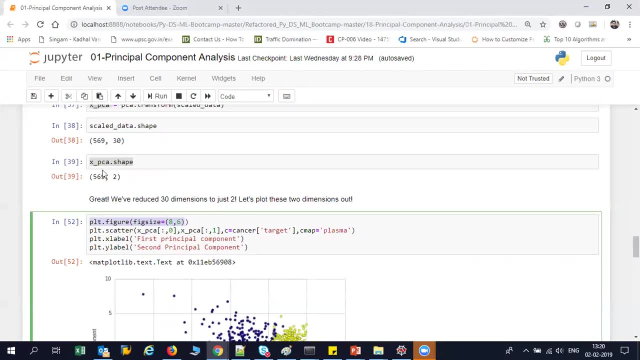 So first of all, I'm going to set up a figure and the figure size is 8, 6.. So 8 is my Width and 6 is my height, and then I am plotting from this X underscore PCA: right, I'm having two features, right? 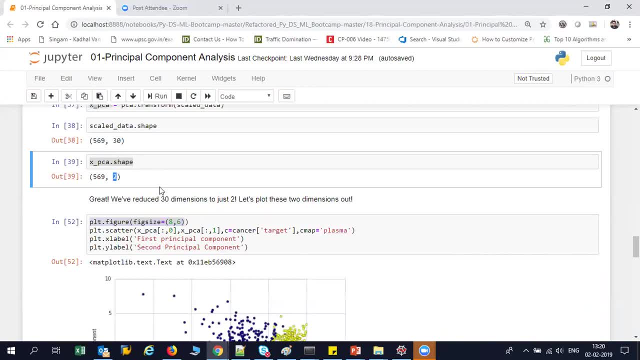 I'm having two features, since I have converted it to two columns, So X, PCA, colon, comma 0 basically means I'm actually retrieving all the details from the 0 index. then, from the first feature, I'm retrieving all the details and my target is basically I'm giving it as cancer of target variable. 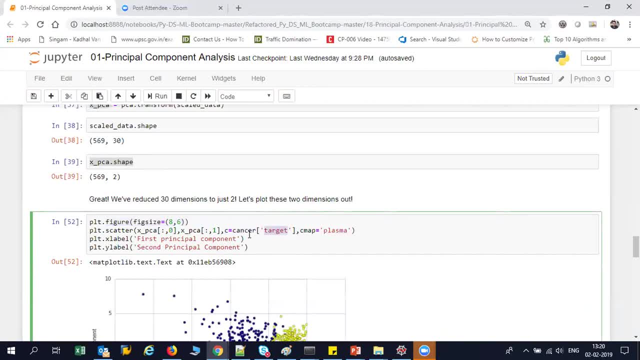 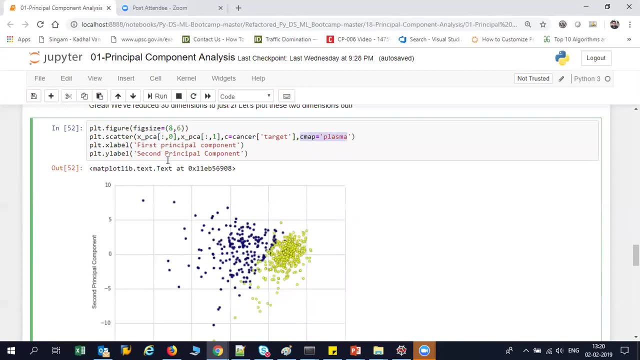 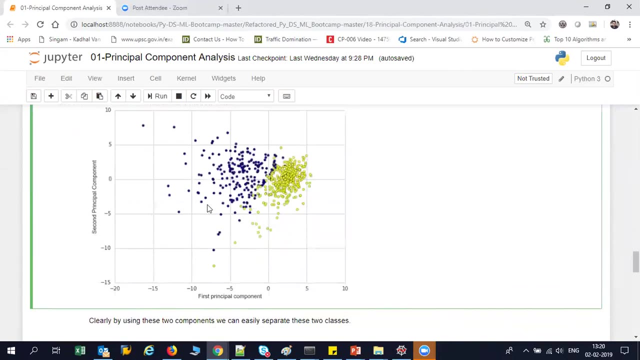 Based on this target. only right, my points will be getting colored. and here I am are going to apply C map just for some style. and In the X label you can see that I've given some title and the Y label I have given some type. Finally, when we try to represent it now, you can see that our data still looks much better, right. 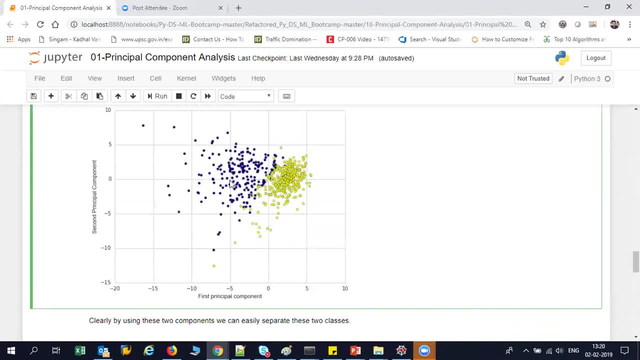 initially just understand, guys, we had 30 dimensions and But now we are just having two dimensions. all these points have got converted into new dimension or scaled into new dimension. Always remember: the first step was what? what was the first step after reading the data set? the first step was: 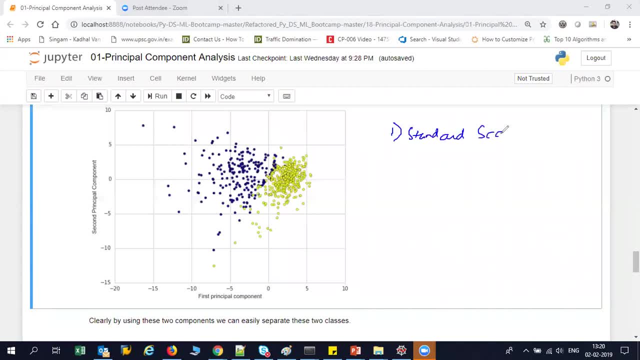 standard scaling, Scaling down right. the second step was basically applying our PC algorithm, in that we did fit and transform. Both. we did fit and transform, but in this, After applying PC, our 30 dimensions has got converted into two dimensions. Now this is how my two dimensions is work. 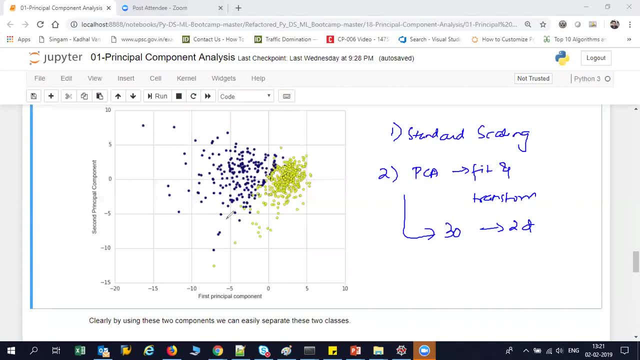 Now you can apply any of the machine learning algorithm. Like, if you apply logistic regression that it is going to create a straight line. the accuracy rate will be very high in this. Okay, but if you use some other algorithms like k nearest neighbor, a nearest neighbor at that time, a. 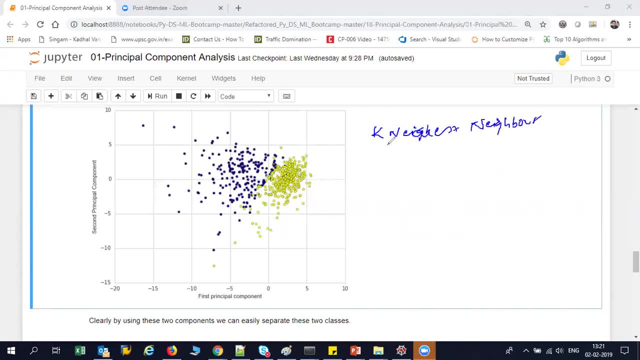 Nearest neighbor at that time. This will also give you a very good accuracy. Otherwise, you can also use decision tree. You can use XG boost. if you don't know about all these things, Guys, please visit my playlist. All the algorithms are there. I've already taken different kind of problems.